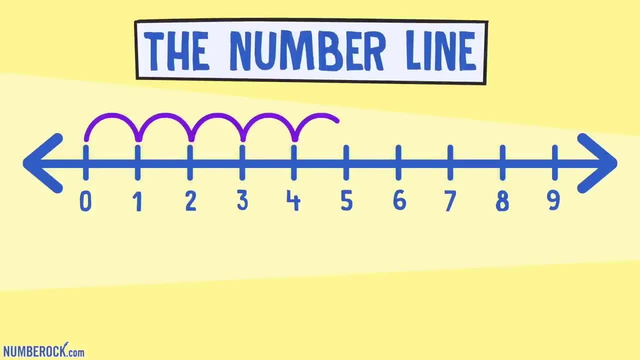 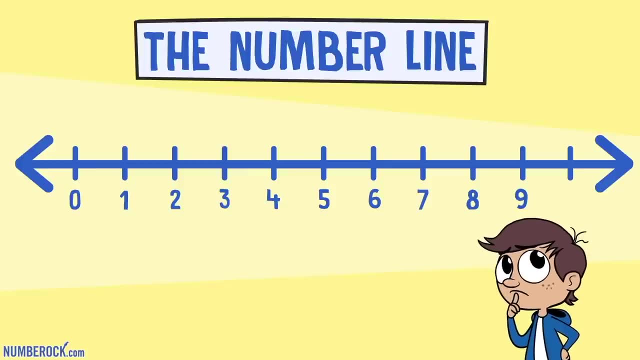 They're represented by lengths and mark, with points spaced equally apart. Now, if we extend this number line one whole number to the right, we'll find The next number that we'll mark is 10.. Now let's extend it again and again. 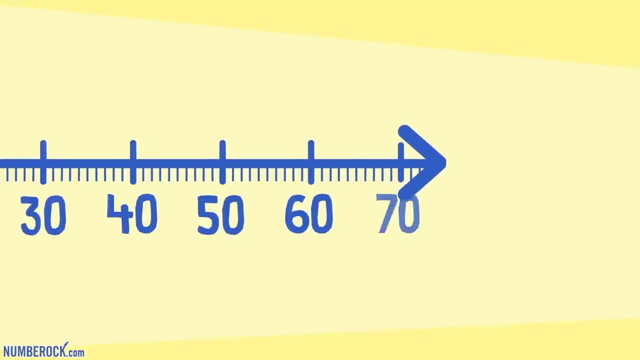 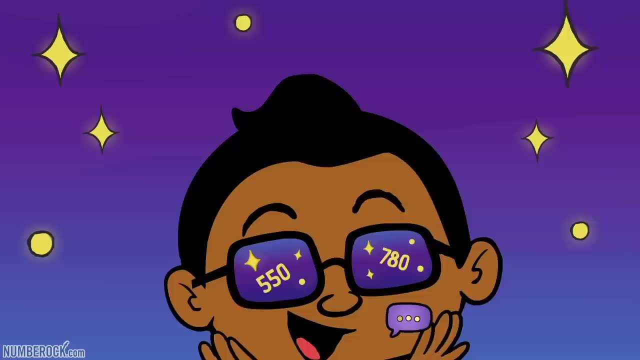 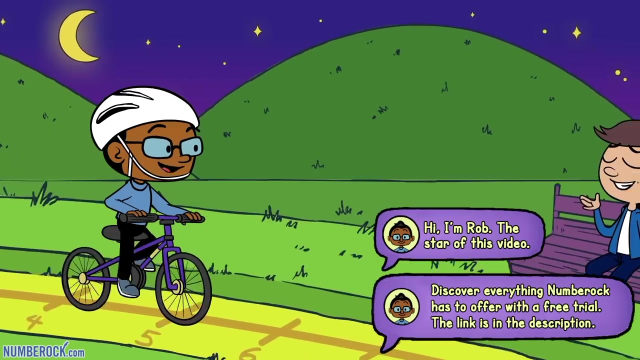 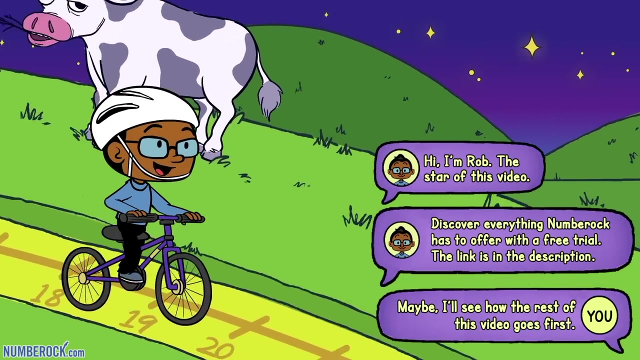 20,, 30,, 40,, 50,, 60,, 70,, 80,, 90. Then my ride ended at 100, but the pattern continues forever ahead. There are many instances when numbers are shown as distances represented on a number line, helping us find sums and differences. 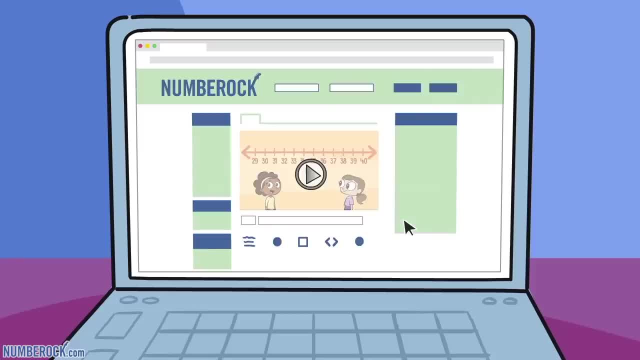 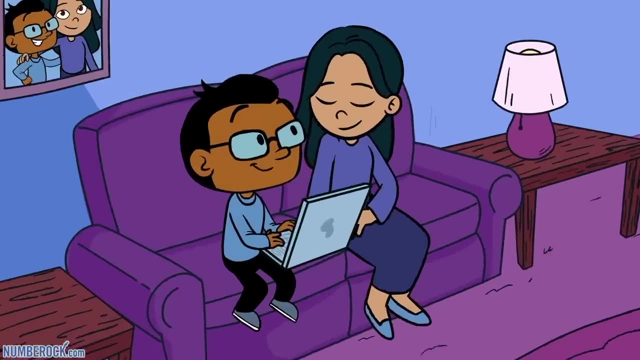 Now Rob's back home hanging out with his mom. They are winding down the day at NumberRockcom. They pick a song about number line skills. a replays their thrills and Rob's mom says: This is chill, We can jump forward on number lines solve problems. 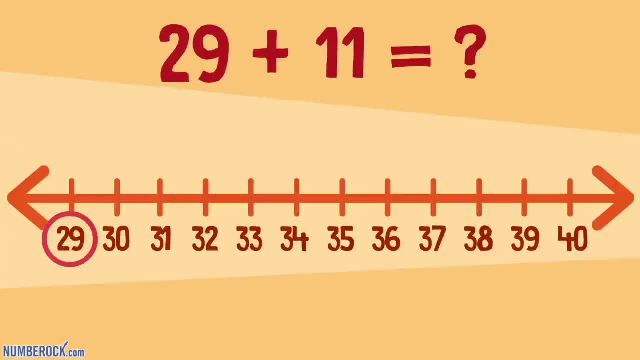 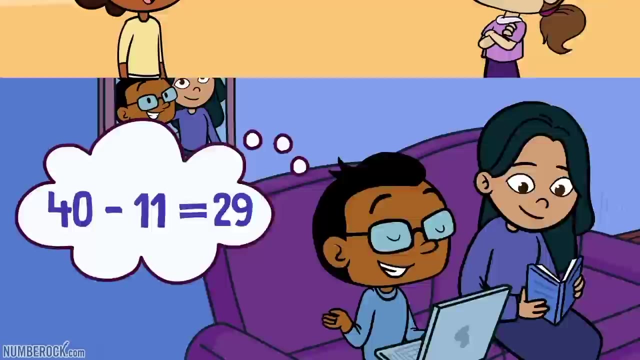 With addition signs. let's add 11 to 29.. Jump one and then 10,, 40's the sum we'll find And we can subtract 11 to rewind, which will take us back to 29.. We can jump backwards on number lines. solve questions with subtraction signs. 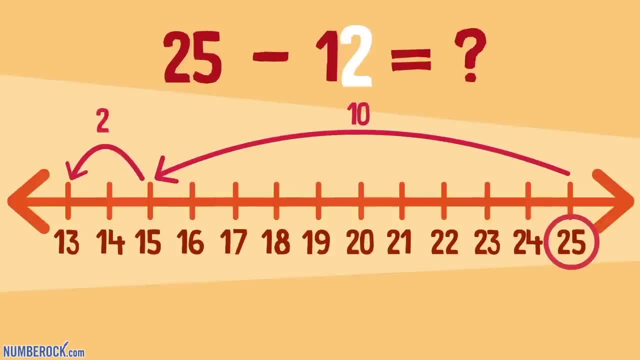 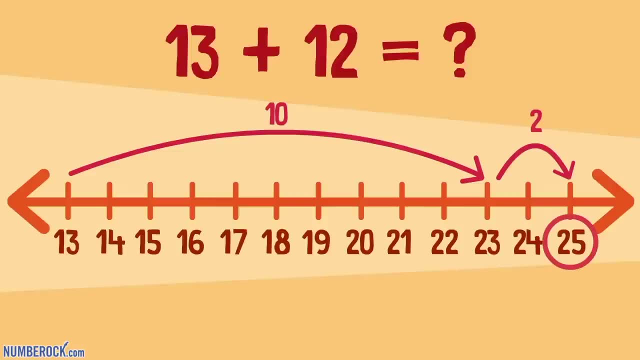 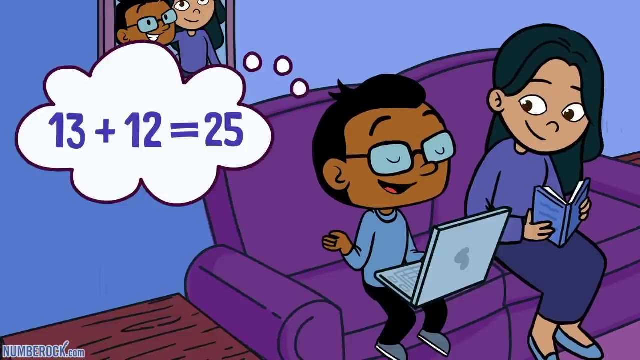 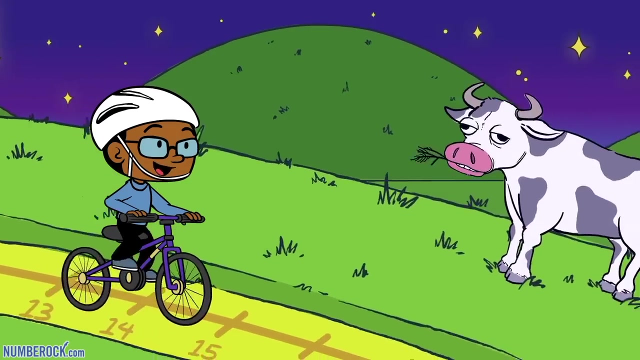 Let's subtract 12 from 25, jump back 10 and 2, 13's the difference we'll find. Now add back 12 to 13, and we will arrive at a sum we've seen 25.. There are many instances when numbers are shown as distances represented on a number line, helping us find sums and differences. 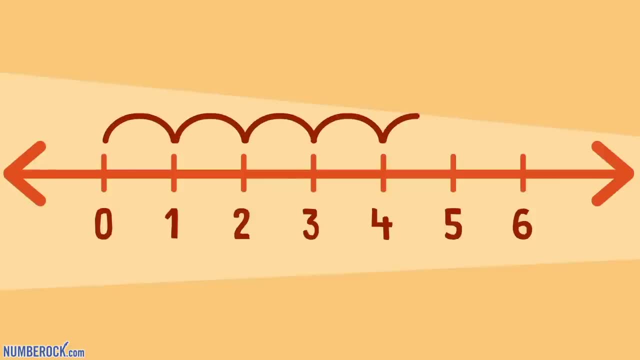 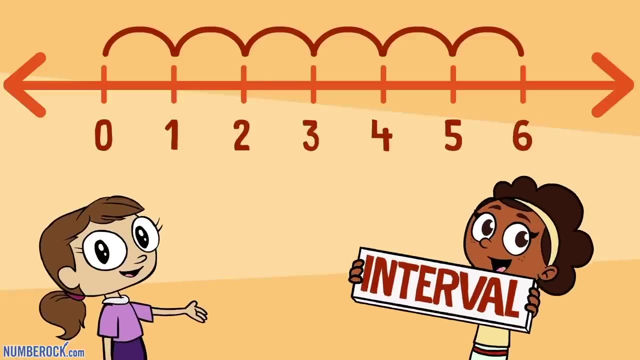 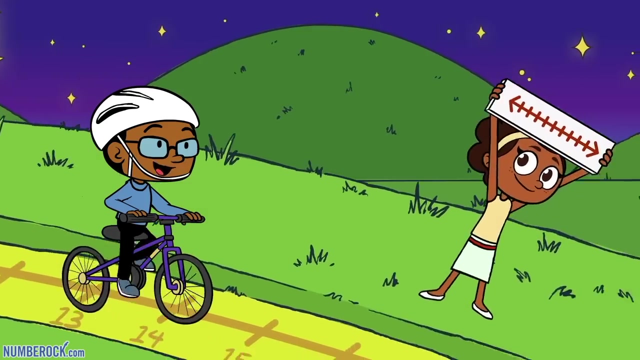 Now here is just one last remark about the distance between each mark. We can call them spaces, but to be technical, their correct mathematical name is an interval. There are many instances when numbers are shown as distances, represented on a number line helping us find sums and differences. 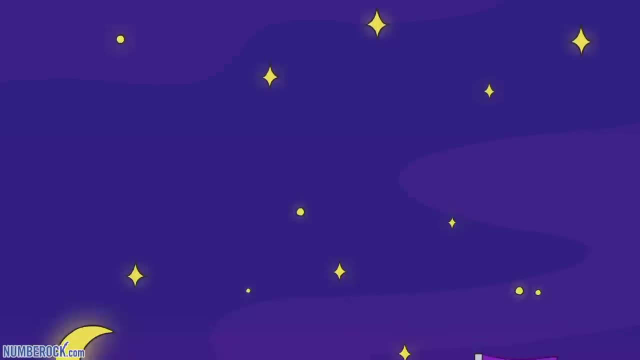 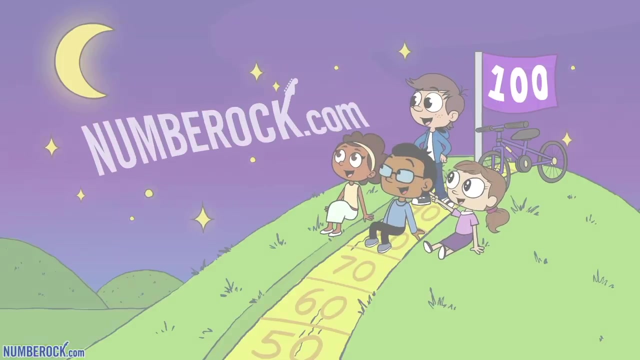 Whoa whoa oh oh, Whoa whoa oh oh, Whoa whoa oh oh. NumberRockcom.